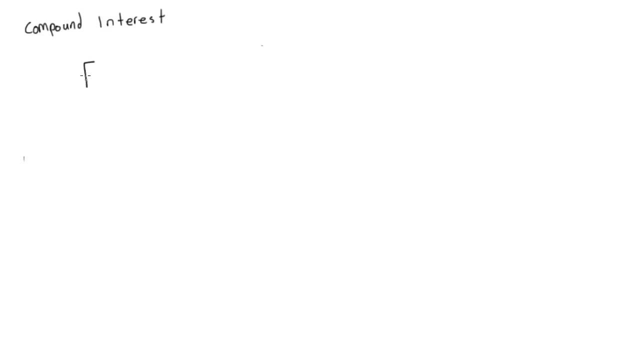 So the formula for compound interest is as follows: We have FV, which is future value, is equal to PV, present value times 1 plus i. This is our annual interest rate, to the power of n, This is our number of years. So I have it here for us. I've already written it down to save you guys. 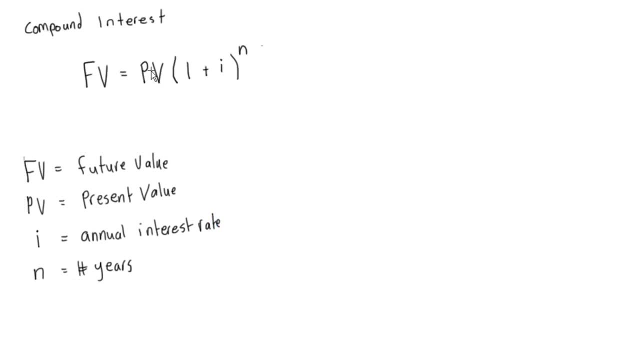 having to watch me write this. So we have future value, present value, annual interest rate and number of years. So basically pretty much any time you ever go to a bank and you want to get a loan or you want to deposit some money into a savings account or something like that, they're. 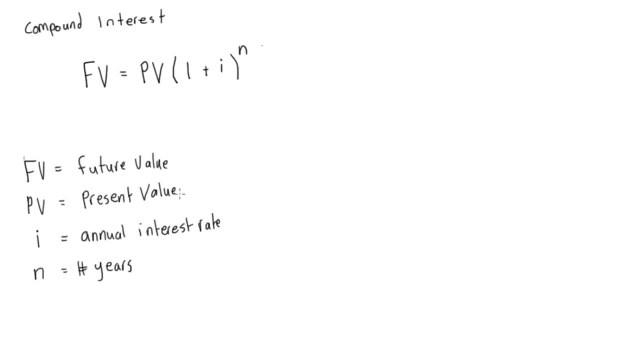 probably going to be compounding your interest annually, unless they say otherwise. So that's this one. We're going to compound interest. So let's say we take $100,000. And we're going to invest this into some bank account that has a 3% interest rate. or again, we 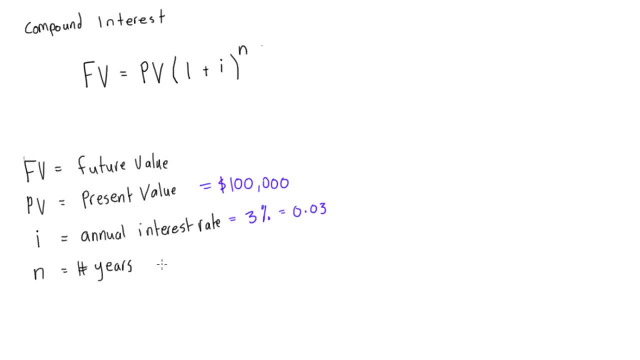 express this in this formula as 0.03.. And we're going to say: we're going to invest this for 10 years. 10 years, All right, So we'll just go ahead and type this into our formula. So our future. 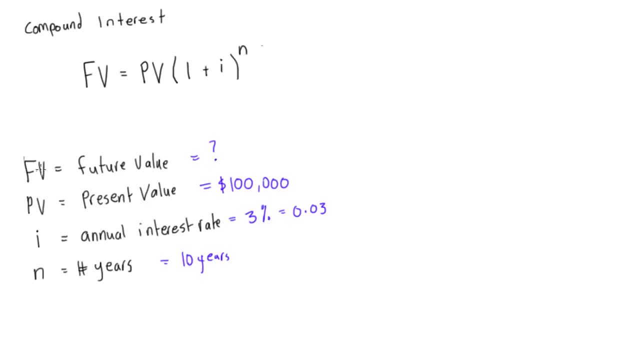 value. this is what we're going to be looking for. We want to know how much money will we have after 10 years. Well, we say that we have. FV is going to be equal to present value is 100,000.. How many zeros do I? 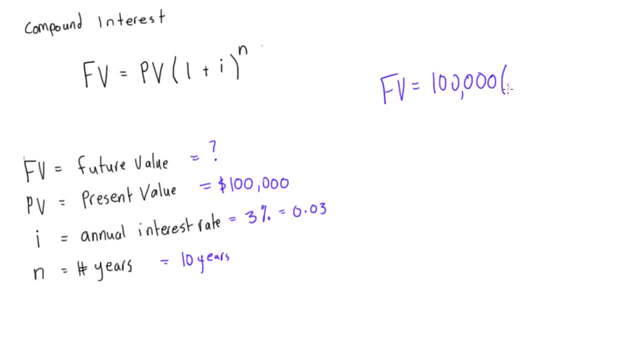 have here 100,000 times 1, plus 0.03 to the power of n, which is 10 years to the power of 10.. So we say that we can have 100,000 times 1.03.. And if you just compute this with your calculator, if you don't have a financial calculator, that's.